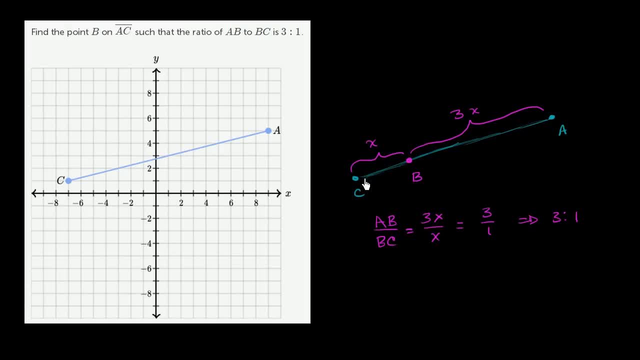 You might be tempted to say, oh well, you could use the distance formula, find the distance, which by itself isn't completely uncomplicated, And then this will be 1 fourth of the way, Because, if you think about it, this entire distance, 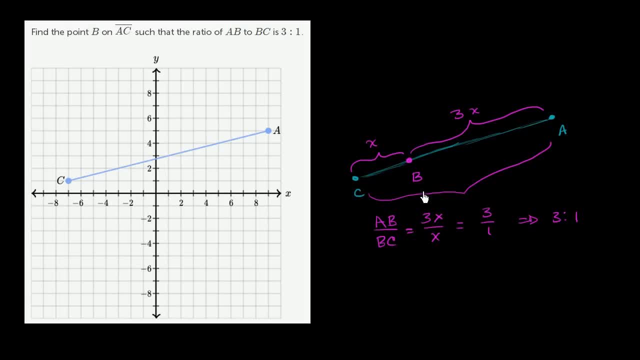 is going to be 4x. This entire distance is going to be- let me draw that a little bit neater- this entire distance, if you have an x plus a 3x, is going to be 4x. So you'd say, well, this is 1 out of the 4x's along the way. 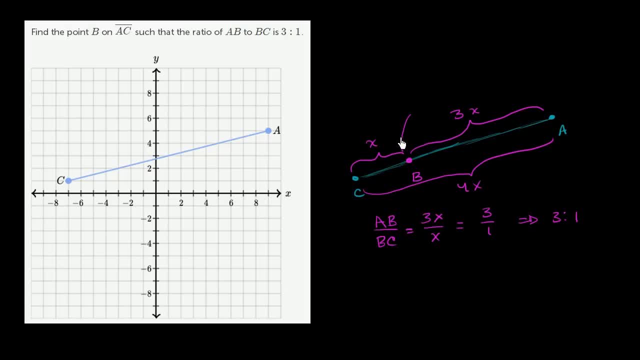 This is going to be 1 fourth of the distance between the two points. So this is- let me write that down- This is 1 fourth of the way between C and B, going from C to A. B is going to be 1 fourth of the way. 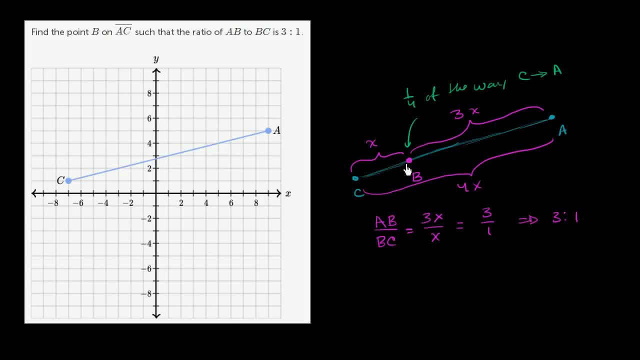 So maybe you try to find the distance And you say, oh well, what are all the points that are 1 fourth of that distance away, but then it has to be on that line. But that makes it complicated because this line 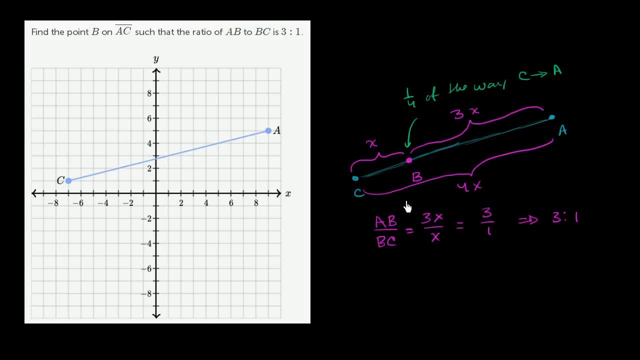 is at an incline. It's not just horizontal, It's not just vertical. What we can do, however, is break this problem down into the vertical change between A and C and the horizontal change between A and C, So, for example, the horizontal change between A and C. 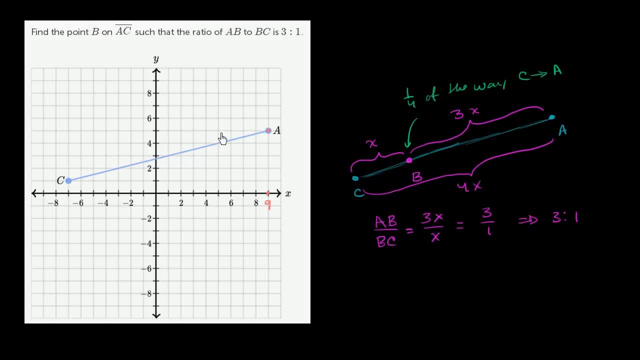 A is at 9 right over here and C is at negative 7.. So this distance right over here is 9 minus negative 7, which is equal to 9 plus 7,, which is equal to 16.. And you see that here, 9 plus 7.. 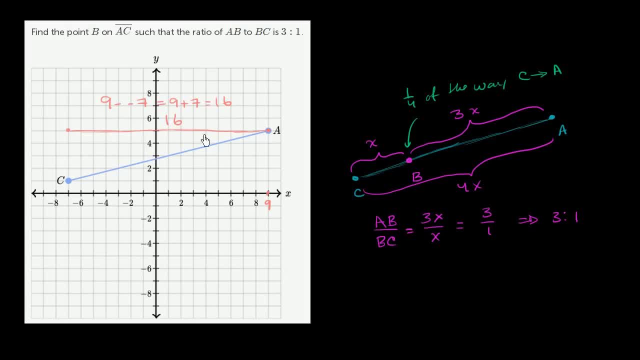 This total distance is 16.. That's the horizontal change- going from A to C or going from C to A- And the vertical change, and you could even just count that that's going to be 4.. C is at 1.. 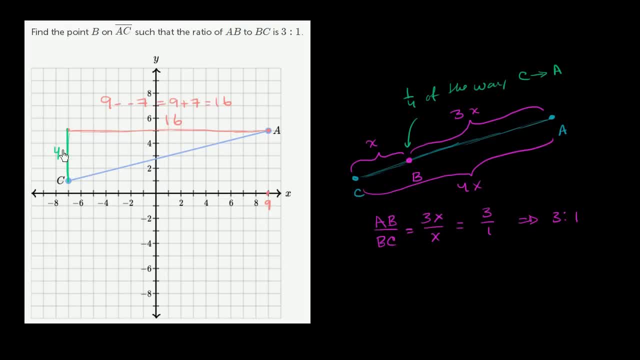 A is at 2.. A is at 3.. A is at 5.. Going from 1 to 5, you've changed vertically 4.. So what we can say? going from C to B in each direction, in the vertical direction and the horizontal direction. 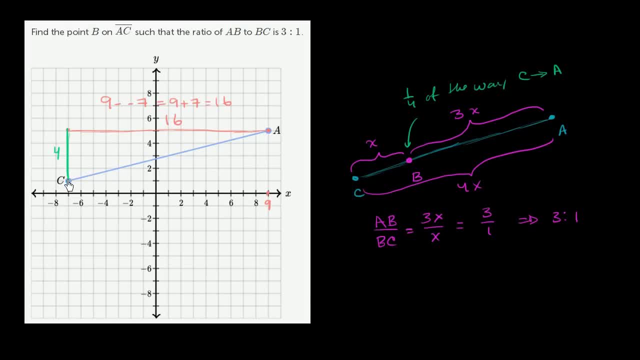 we're going to go 1 fourth of the way. So if we go 1 fourth in the vertical direction we're going to end up at, y is equal to 2.. So I'm just starting at C, 1 fourth of the way.